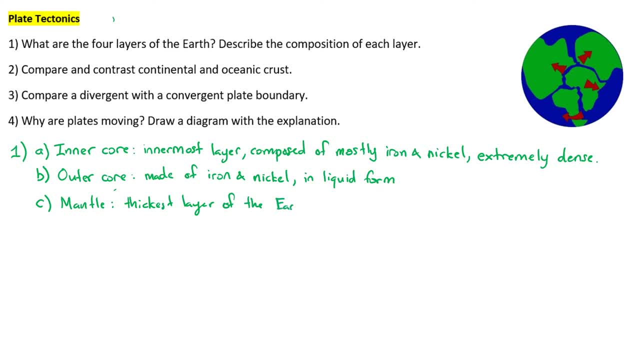 Earth which is above the core, containing magma, Magma. Nod to Austin Powers there. And then another point is that it contains the asthenosphere, which is the outer part of the mantle, Composed of semimoltan ductile rock. 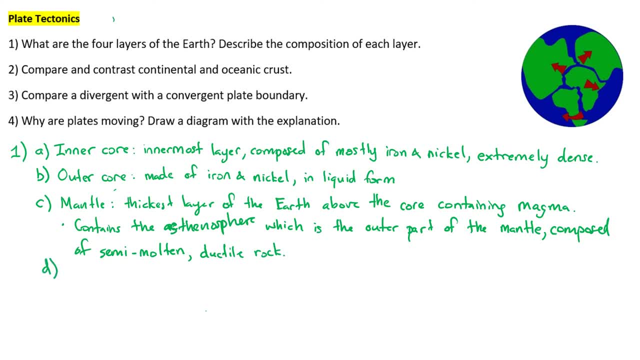 And then we have the crust. The crust is extremely thin, cold and brittle compared to what lies below. The crust is made of relatively light elements, especially silica aluminum. It is an oxygen. Another name for it would be the lithosphere Number two. compared contrast continental and oceanic crust. 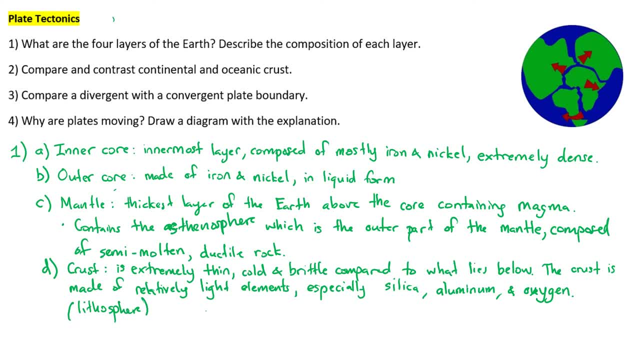 I'm going to write it right here: They both float on top of the mantle. okay, continental crust. I'm just gonna write down: continental is less dense. and then we have, let's just say that is less dense than oceanic crust. compare a divergent with a. 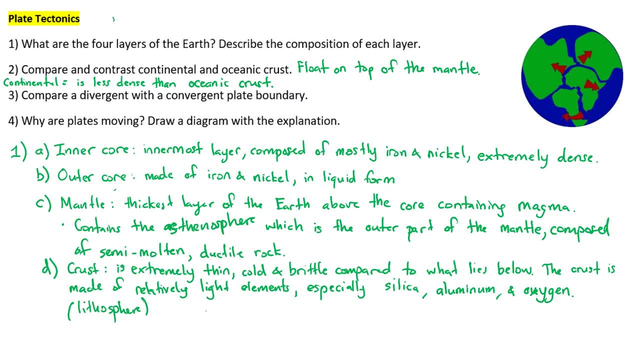 convergent plate boundary, so divergent. y'all right here divergent where plates pull away from each other, forming my old earthquakes and volcanoes as magma comes to the service. and then i'm going to write over here: 下面 of those under four is truly, truly under three. it is the convergent, so convergent. 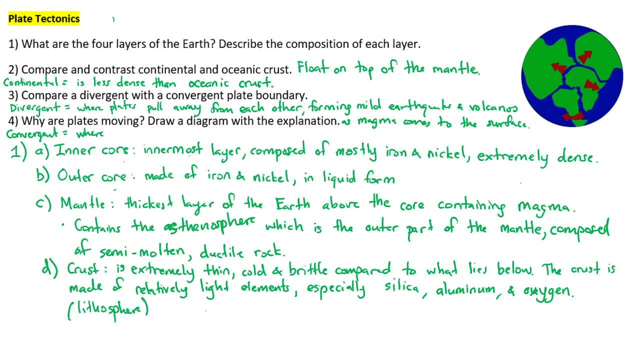 boundaries are where two plates are pushing into each other and, based on their density, y'all different things occur. so one plate is more dense than the other. the less dense plate gets subjected under the more dense plate, but if they're both very, very low density plates, they form mountains, like the. 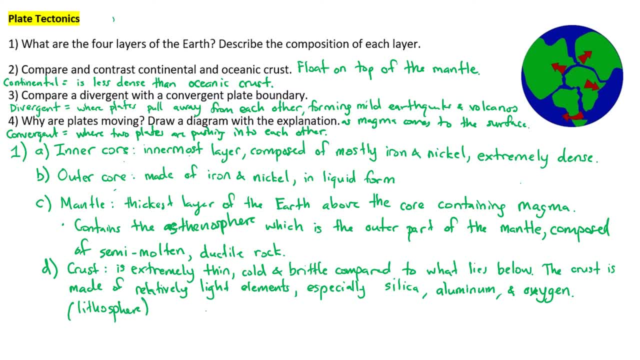 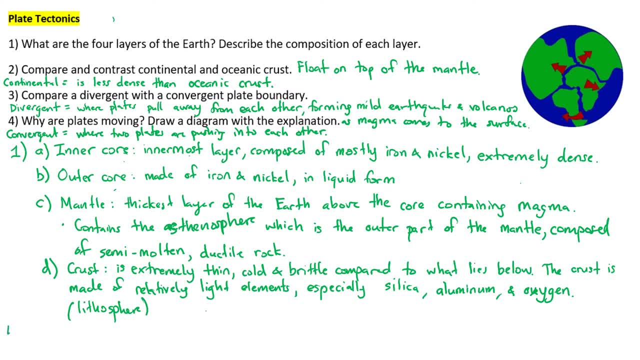 don't know. I don't know. the diagram will be very small because I'm running on a room here, but we have number four in this space. so plates on our added planet's surface move because of the intense heat and the earth's core- so let's write that down- move because of 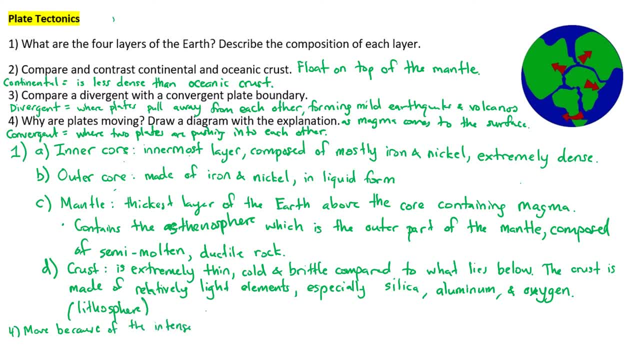 the intense heat in the earth's core that cause molten rock in the mantle to move. it moves in a convection. so warm materials, warm materials, materials, warm materials rises, and then we have cool sinks, and then we have cool sinks, and then we have cool sinks and the picture for number four I'm gonna. 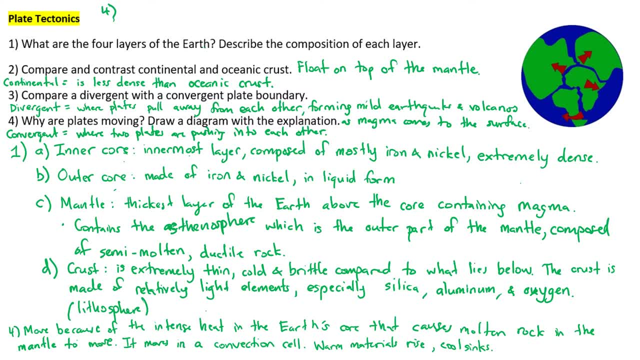 and the picture for number four, I'm gonna. and the picture for number four, I'm gonna. draw it right here we have the core. draw it right here. we have the core. draw it right here. we have the core, and and And, then the mantle, and within the mantle we have those convection currents. 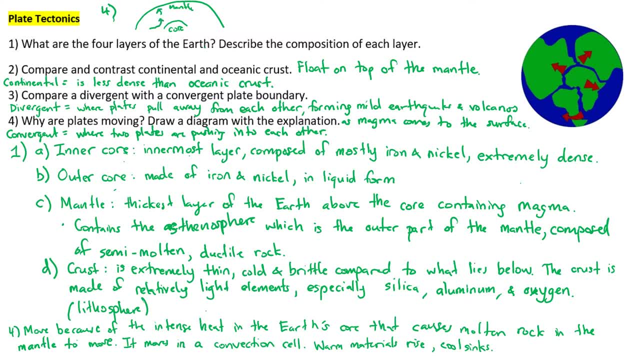 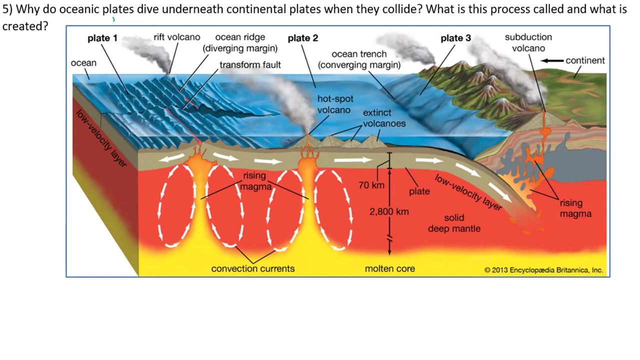 So hot rise and then cool sinks, And that's what causes the plates to move. Those plates are floating on top. so again, that's what causes the crust to move. Number five: why do oceanic plates dive underneath continental plates when they collide? 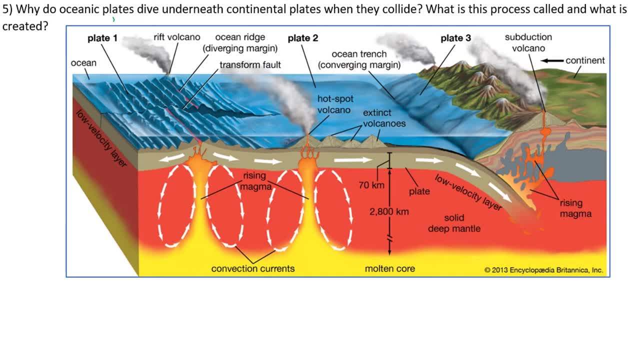 What is this process called and what is created? So we have oceanic plates that are more dense than continental plates, causes them to dive underneath when they collide. Number six: why do oceanic plates dive underneath continental plates when they collide? 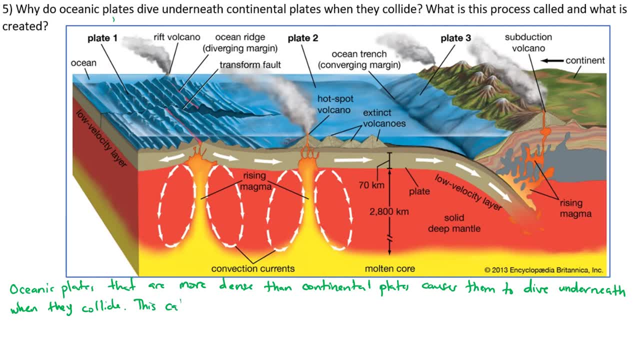 This is called, What is this process called and what is created? Number six: why do oceanic plates dive underneath continental plates when they collide? A convergent boundary, specifically subduction, is usually created in a flip of land, resulting in mountain ranges. 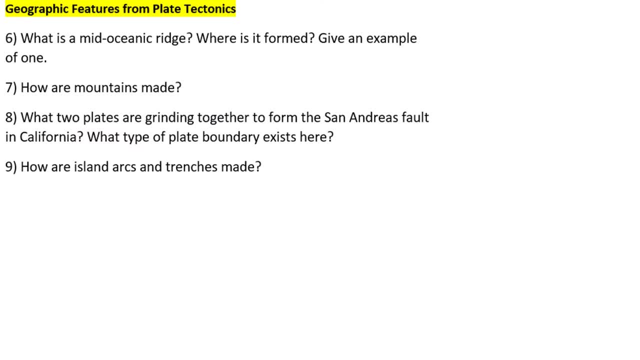 What is a mid-oceanic ridge? Where is it formed? Give an example of one. So the mid-Atlantic ridge is simply one sea floor spreads at a great depth in the ocean from a divergent plate boundary. So the example would be the Mid-Atlantic Ridge. 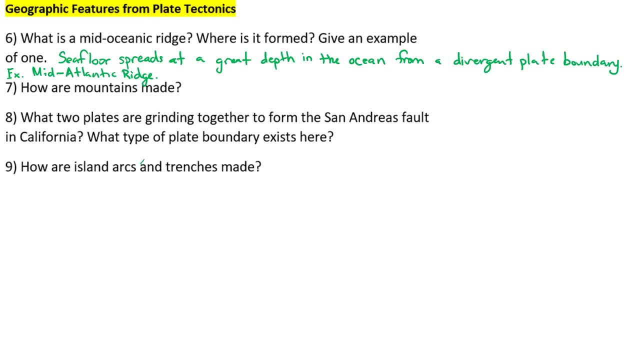 How are mountains formed? So mountains are made at convergent Plate boundaries where two plates collide. Number eight: What two plates are grinded together to form the San Andreas Fault in California? What type of plate boundary exists here? So the Pacific? 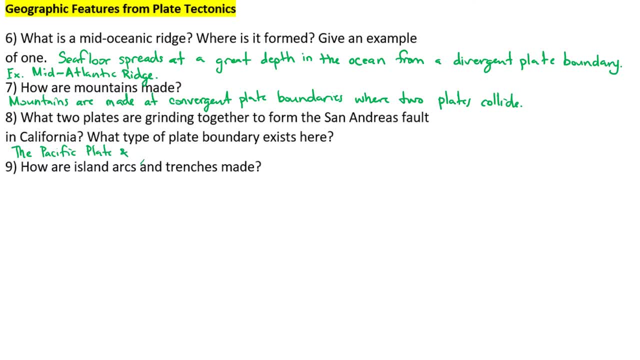 Plate And the North American plate. This is a transformed plate boundary. How are island arcs and trenches made? An island arc is a chain or group of islands that form from From From, From From From. This has volcanic activity along a subduction zone. 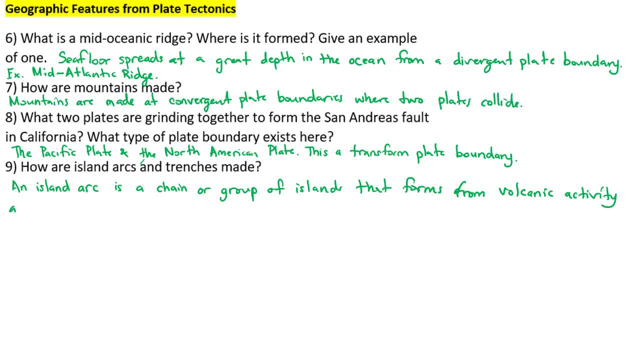 Subduction occurs when an oceanic lithosphere salmon, When a seism��면 oceanic lithosphere Diesel. Al tie a cat in here. Her sinks underneath continental or another oceanic lithosphere. Trenches are formed by subduction, a geological process in which two or more 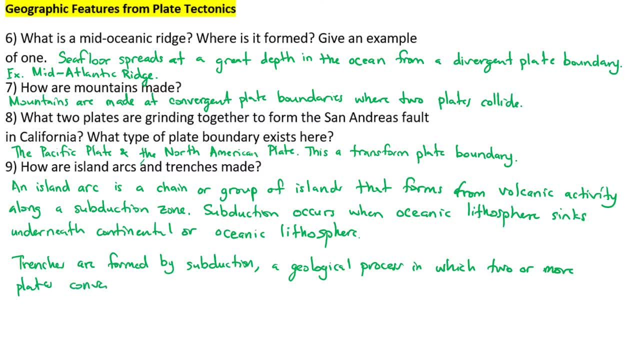 plates converge and the older denser plate is pushed beneath the lighter plate And deep into the mantle, causing sea floor spreading, Oh no sorry, Causing the sea floor and outer most crust to bend. And the older denser plate is pushed beneath the lighter plate. 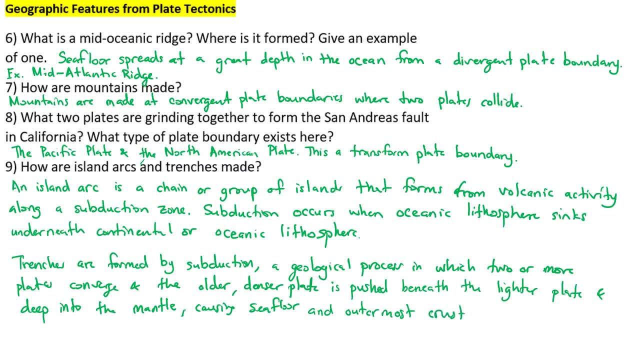 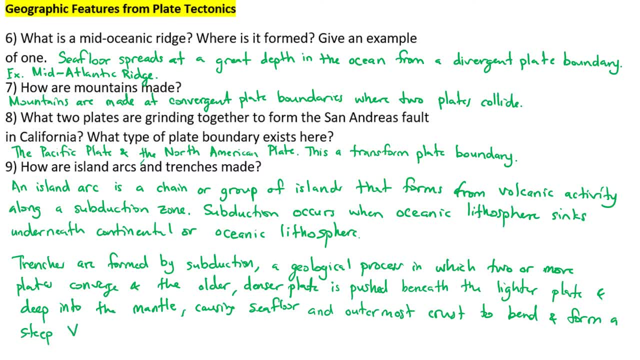 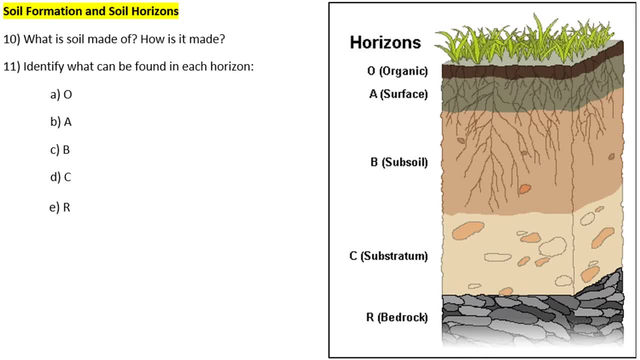 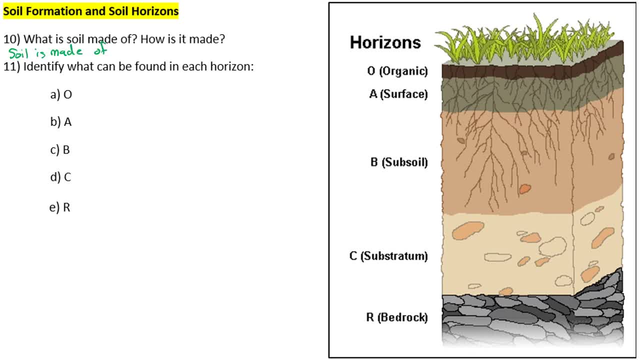 And deep into the mantle, causing sea floor spreading- And deep into the mantle, causing sea floor spreading- of a mixture of organic matter, minerals. I'm going to write it up here: minerals, gases, liquids and organisms that together support life. 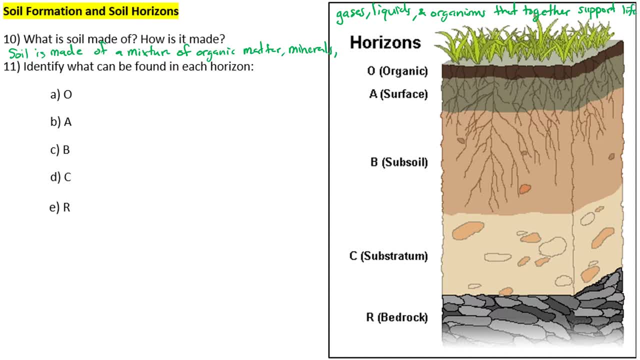 I'm going to write underneath the second part of it. how is it made? as formed from physical matter, And chemical weathering of rocks Identify what can be found in each horizon. So for the O horizon, it is the organic matter in various stages of decomposition. 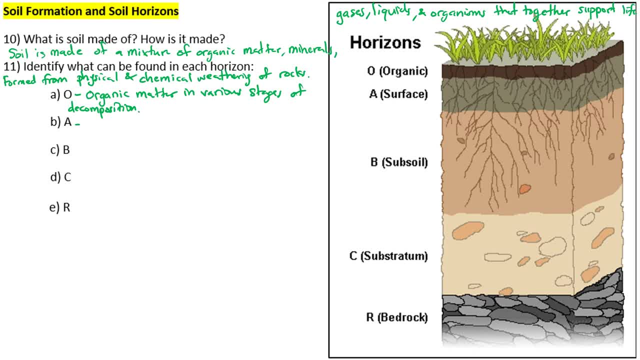 So the O horizon is made of all the materials that are linked together. A would be a zone of underlying organic material mixed with underlying organic material mixed with underlying organic material. B- zone of accumulation of metals and nutrients. C would be the least weathered portion of soil. 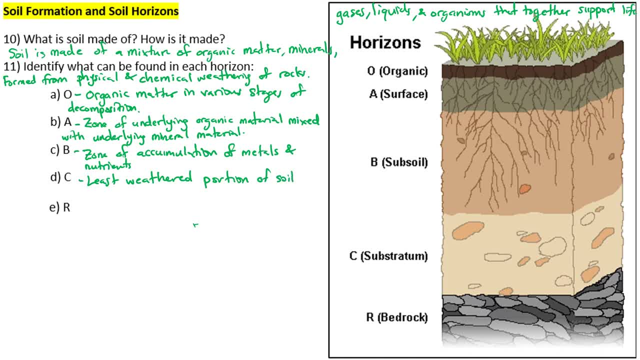 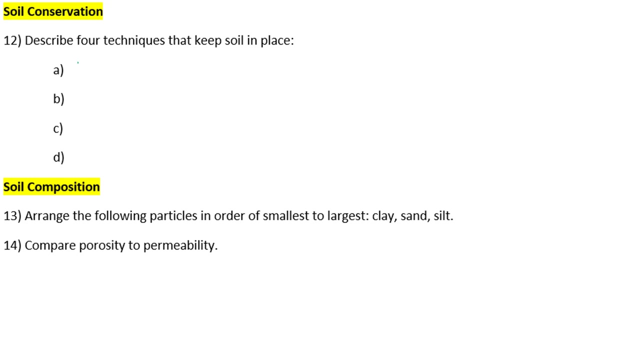 Very similar to the parent material. And then R is basically the layer of unweathered or partially weathered bedrock. Describe four techniques that keep soil in place. So we have contour plowing. And then contour plowing is plowing grooves into the desired farmland. 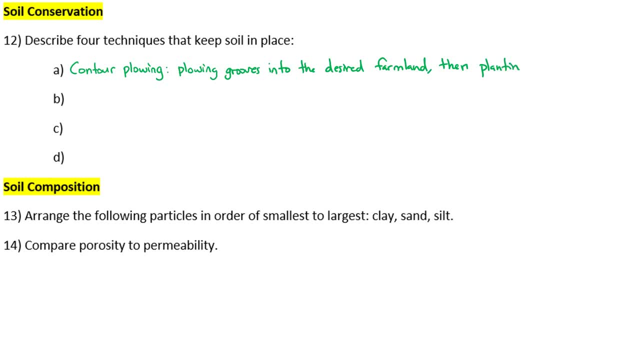 Then planting the crop furrows in the groove and following the contours, We have the windbreaks. Rows of tall trees are used And dense patterns around the farmland. Okay, And prevent wind erosion. No-till is a method of growing crops year-round. 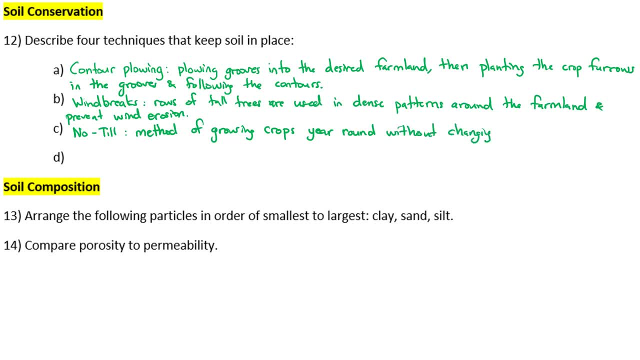 Without change: Okay, By changing the topography of the soil by tilling or contouring, And then cover crops- Okay, And we can use this to cover crop three, four or five years- Okay, And then we can also use this method to help contribute to the development. 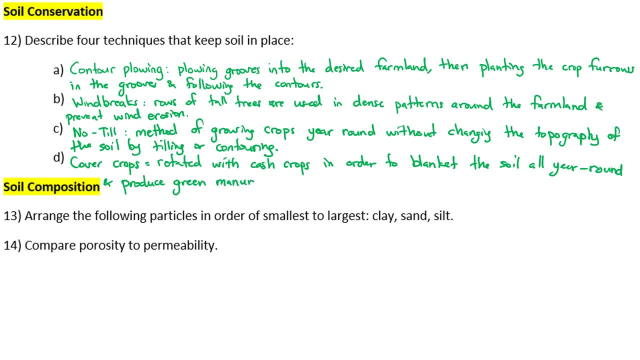 Okay. Of trees, Yes, And then we can use this method, Yeah, To raise crops and to help grow the soil, And then, after the tilling, we can use this method, Okay, And then we can also use this method to add soil. 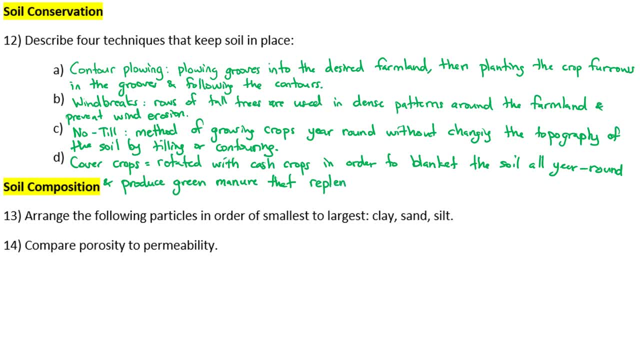 Okay, So we can add soil. Okay, So we can add soil. Okay, So we can add soil. replenishes nitrogen and other critical nutrients. 13 arrange the following particles in order of smallest to largest: clay, sand and salt. so clay silt. 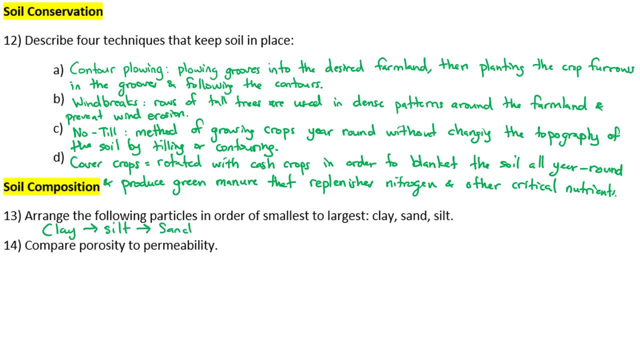 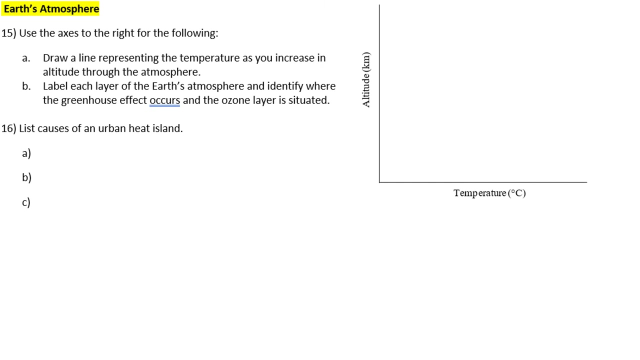 then sand. 14. compare porosity to permeability: porosity, measure how much a rock is open space, and then permeability, and then permeability, a measure of the ease with which fluid can move through a porous rock. So use the axes to the right for the following: Draw a line representing the temperature as you increase. 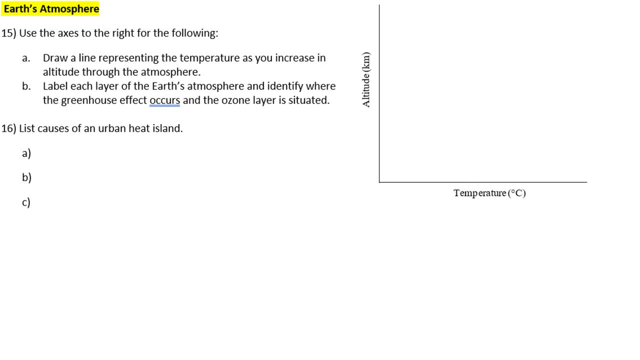 in altitude through the atmosphere, Label each layer of the atmosphere and identify where the greenhouse effect occurs and the ozone layer is situated. So we have the curve here. the line approximating the values slight goes up halfway here it goes up, then it gets close to here it goes. 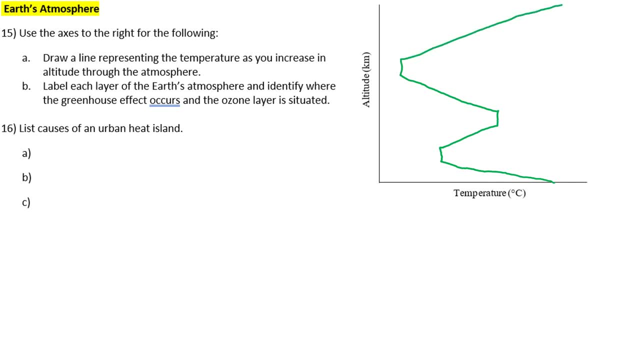 up and then, exponentially, temperature goes haywire out. Okay, so the layers. now I'm going to draw it in a different color. We have this separation and this would be the troposphere. Then, at the other end, this middle area is the stratosphere. 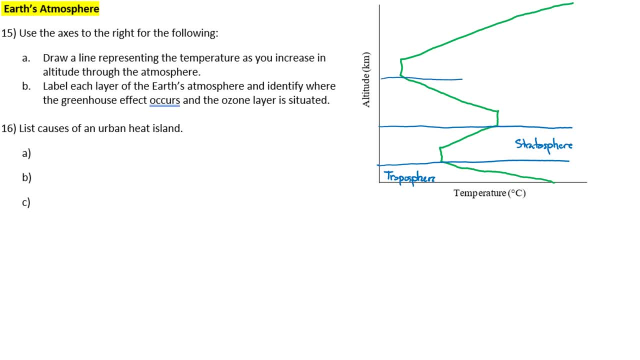 And we have another layer here, and this is the mesosphere, And the last one, y'all, the thermosphere. Okay, so, with that said, the ozone layer is situated in the stratosphere, y'all. So ozone layer, Greenhouse effect, occurs within the troposphere itself. 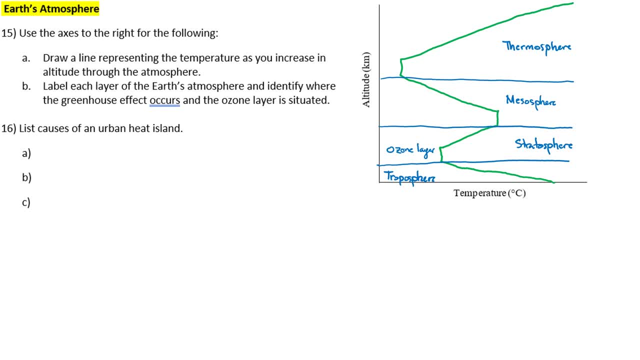 So we say, in light moments, if the season, tools of wave and exoplanets, Okay, number 16.. List causes of an urban heat island. So causes y'all changed or change in surfaces of urban areas, waste, heat, and then population density, more people, more body heat there. 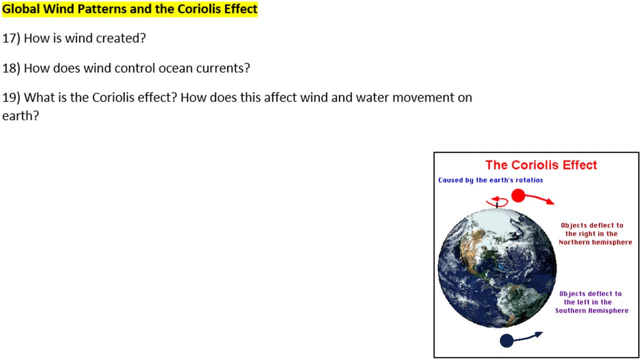 17: how is wind created? so it is produced by the uneven heating of the earth's surface by the sun. number 18: how does wind control ocean currents? so i'm going to write 18 right here for more room for my answer. these surface currents are. 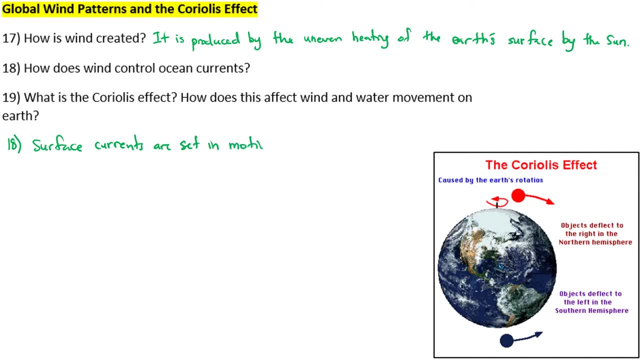 set in motion by the wind, which drags on the surface of the water as it blows. the winds pull surface water with them, creating currents. number 19: what is the coriolis effect? how does this affect wind currents effect, wind and water movement on earth. so 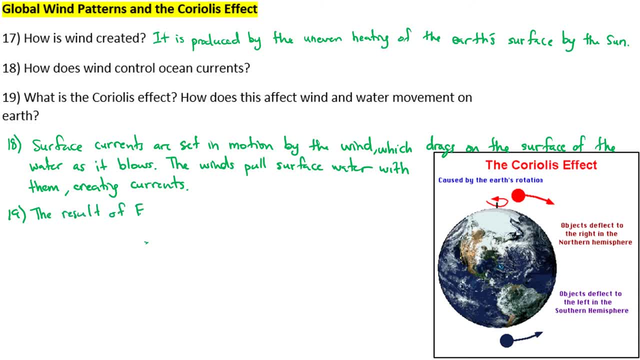 it is the result of earth's rotation on weather patterns and ocean currents. the coriolis effect has a power of 20, as we have seen in our previous example. the coriolis effect is a power that allows the air to flow through the atmosphere and the atmosphere. 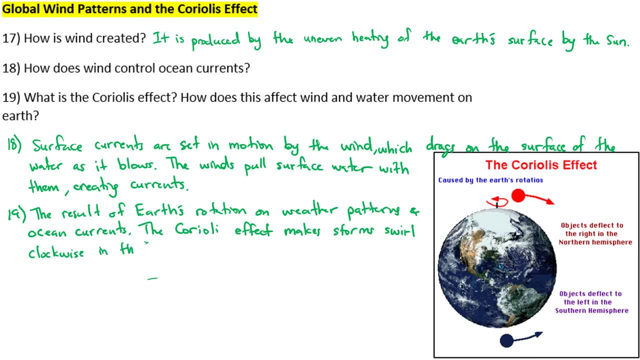 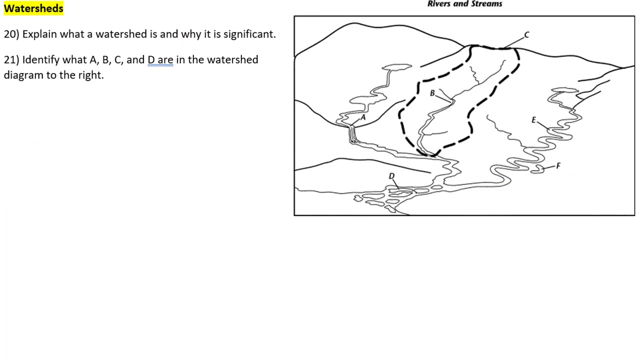 produces air and the air makes storms swirl, clockwise in the southern hemisphere and counterclockwise in the northern hemisphere. explain what a watershed is and why it is significant. so I'm gonna be answering it here. 20 watersheds are important because the surface water features and storm water runoffs within. 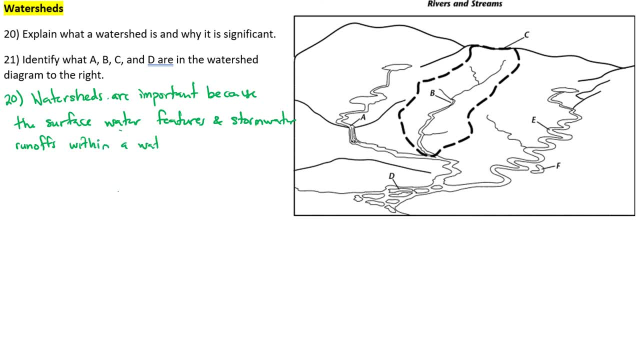 a watershed ultimately drains to other bodies of water. it is essential to consider these downstream impacts when developing, when developing and implementing water quality protection and restoration actions. so next we're gonna identify what a, B, C and D are in the watershed diagram, so I'm gonna label it within it, y'all. so a is the waterfall. 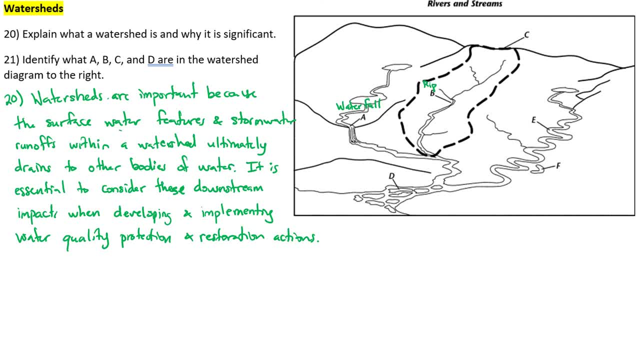 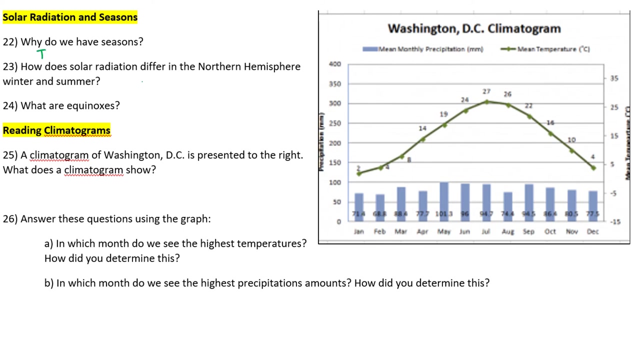 B is the rip-pairing zone, C is the water fall zone, D is the rip-pairing zone, C is the water fall zone, D is the water fall zone would be the ridge and d is the estuary. why do we have seasons? so it's simply due to the tilt of the earth's axis, and the rotation around the Earth's axis on itsCome. to think of eigentlich an everything would be depending on the size of the Earth's axis, but as long as the location of the Earth's axis is parallel to the point B of the Earth's axis and the wrecker pelt would be parallel to the point C of the Earth's axis. 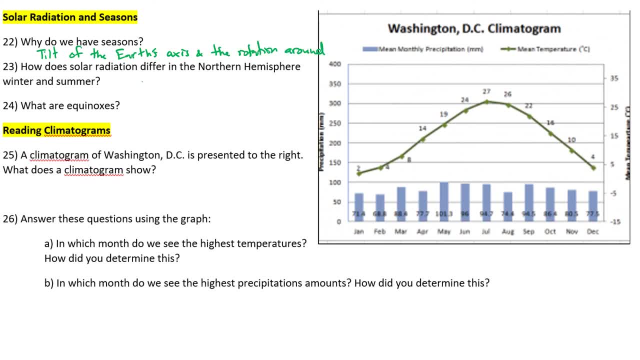 So why are we seeing seasons And why is that? It seems HiAM gonna be so plate. a little bit earth. the Sun 23. how does solar radiation differ in the northern hemisphere winter and summer? so when the North Pole of Earth is tilted toward the sun, we in the northern hemisphere 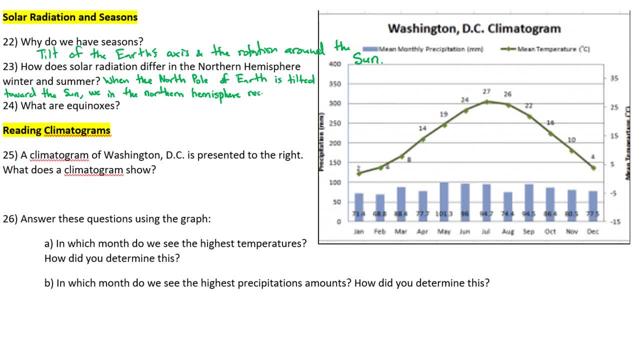 we in the northern hemisphere. we in the northern hemisphere receive more sunlight, and that word is sunlight, y'all apologize. Sun light and it's summer 24, or? let's continue with that. we didn't finish. I'm gonna answer it part two, right here. when it is tilted away from the Sun. 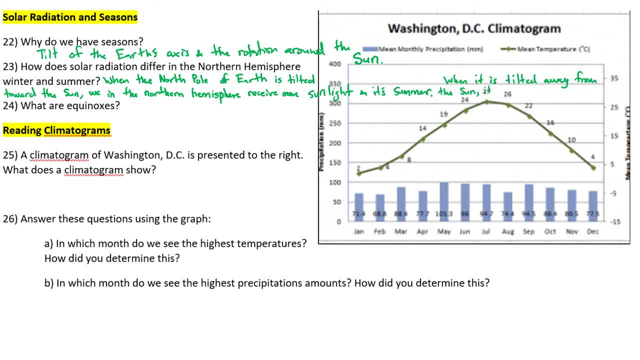 it is winter in the northern hemisphere. okay, 24, what are the equinoxes when day and night are equal length? so when it is tilted away from the Sun, it is winter in the northern hemisphere. so reading climatograms, so we have number 25, a climatogram of Washington DC. 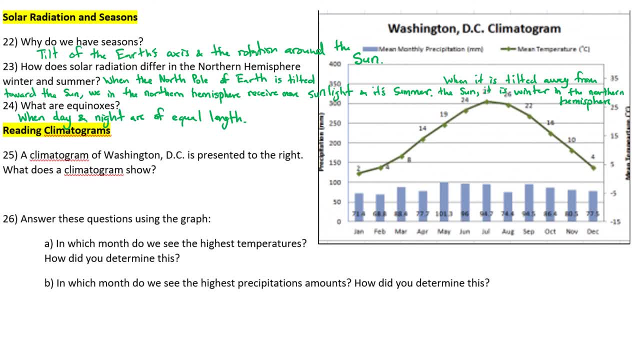 is presented to the right. what does a climatogram show? so it shows the mean temperature. mean is just the average temperature and average rainfall over the course of a year. number 26 a: in which month do we see the highest temperature? so this would be July. 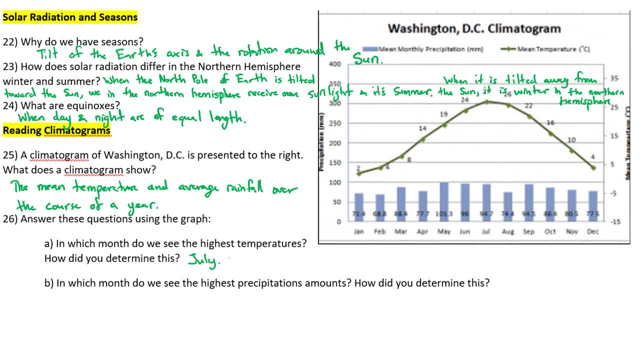 VE average. we can determine this by looking at the line graph. in which month do we see the highest precipitation amounts? so this one would be in May, and we look at the bar graph. bar graph per month and a few months set props in these two modes. well, we can determine this by looking at the sign. this is April in 2022. cameras and Erdman app- it's called Mr Thomas Carson surveillance. an achievement start at 5: Groاm. 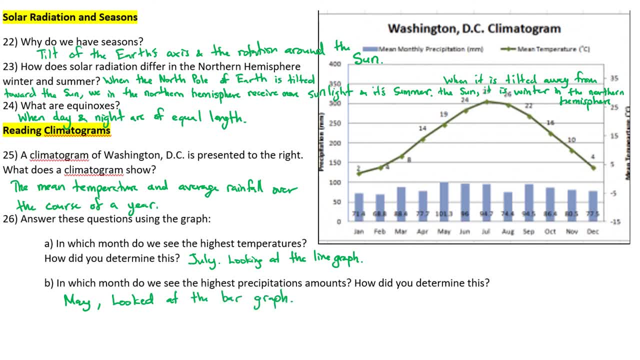 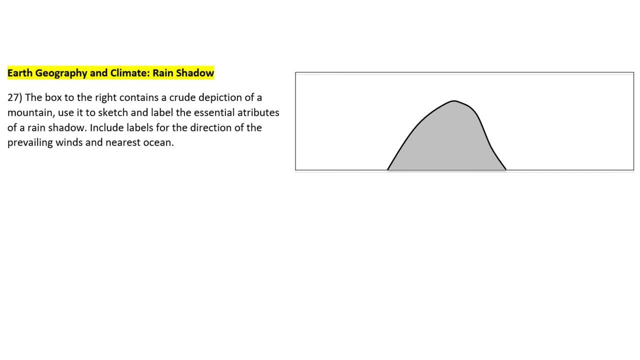 not in the YouTube description up 27. the box to the right contains a crude depiction of a mountain. use it to sketch and label. the essential attributes of a rain shadow include labels for the direction of the prevailing winds and nearest ocean. so I'm gonna be labeling it here. y'all, I'm not a big. 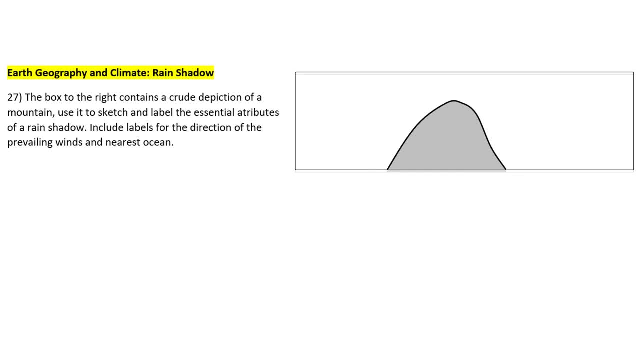 artist, but I'm gonna try my best. so we're gonna label the sea level. okay, make it too big. they're gonna have land here. so this is the sea level. we have the prevailing winds, and this is called the windward side, okay, and then we have clouds. 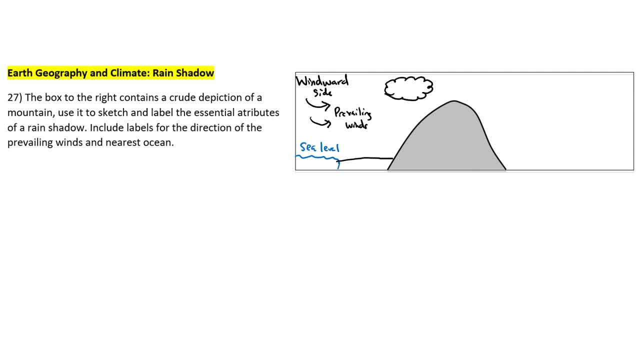 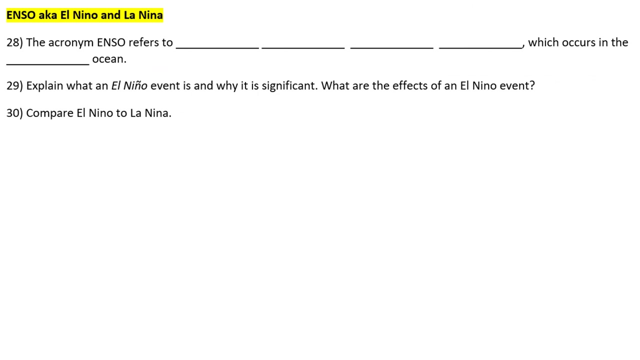 with rain, and then on the other side we have the leeward side, so the rain shadow. dun-dun-dun the acronym, and so refers to El Nino, southern oscillation which occurs in the Pacific Ocean. explain what an El Nino event is and why is significant are the effects of an El Nino event? so I'm gonna lay, I'm. 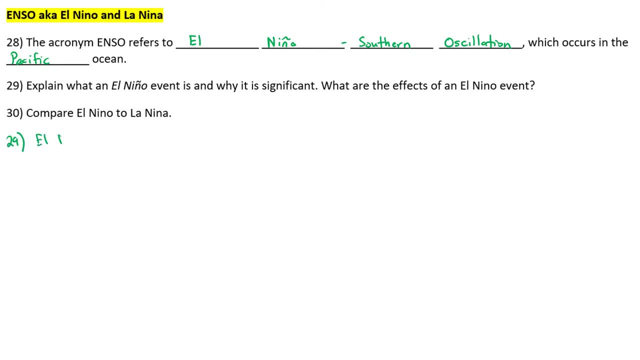 gonna answer it down here y'all. so El Nino is a climate pattern that describes the unusual warming of surface waters in the eastern equatorial Pacific Ocean. this has negative impacts off the coast of South America because it stops the upwelling of the cool, nutrient-rich water, which decrease the amount of fish available for. 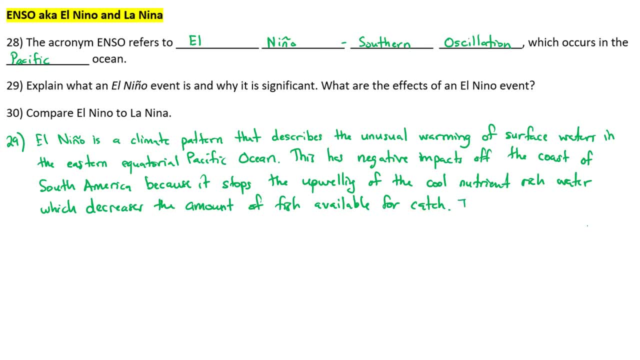 catch. this also can increase storm systems in South America. El Nino can also lead to unusually high temperatures and reduced rainfall in Australia, and then we have 30. compare El Nino to La Nina. so El Nino whoa. El Nino is the warming of surface water. 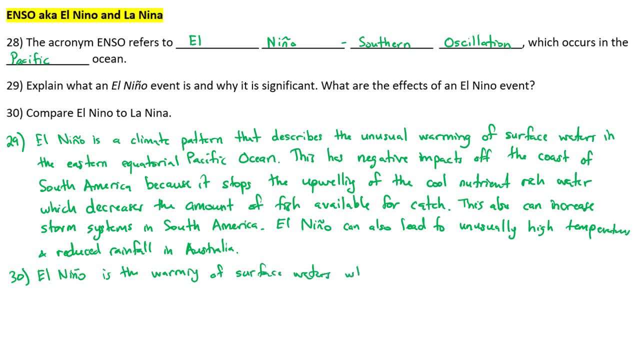 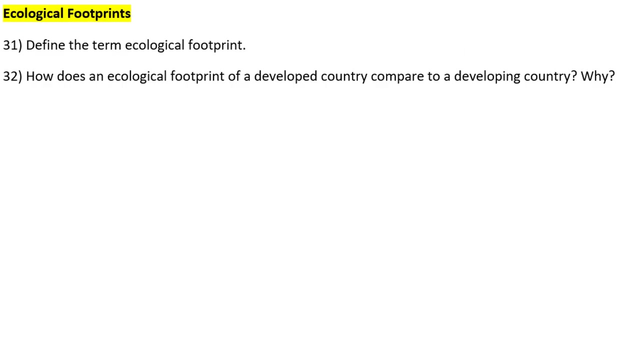 while La Nina is the cooling surface water. okay, define the term ecological footprint, so I'm gonna write it right here: the impact of human activity measured in terms of of the area of biological productivity, productive land, apologies and water required to produce the goods consumed and to assimilate. 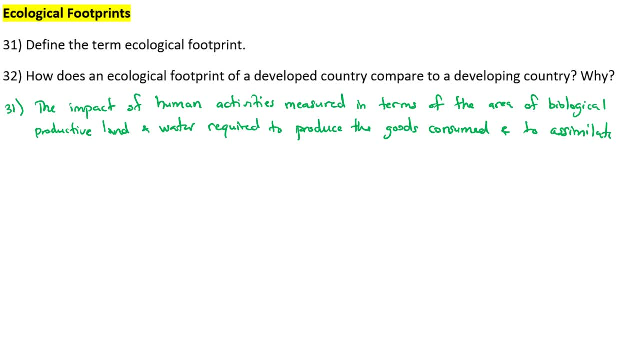 the waste generally generated. so 32: how does an ecological footprint of a developed country compared to a developing country, and why so higher income? more developed countries- generally more developed- have a higher footprint than poor, less developed countries. this is mostly times Due to the higher energy and food demands of developed countries. 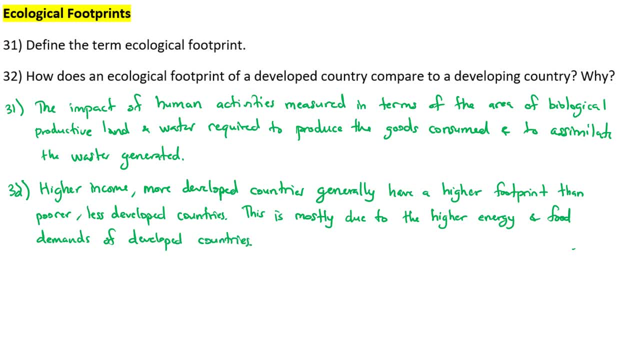 Okay, so that is it for today. Have a good one y'all.